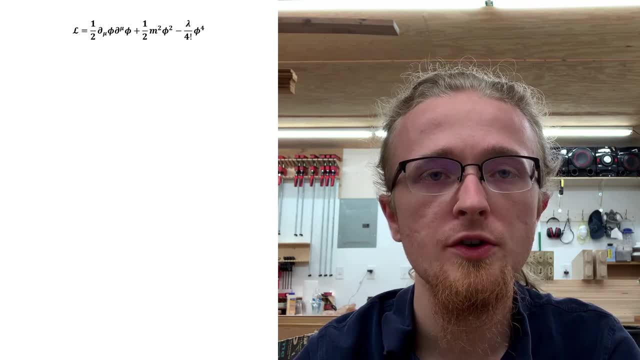 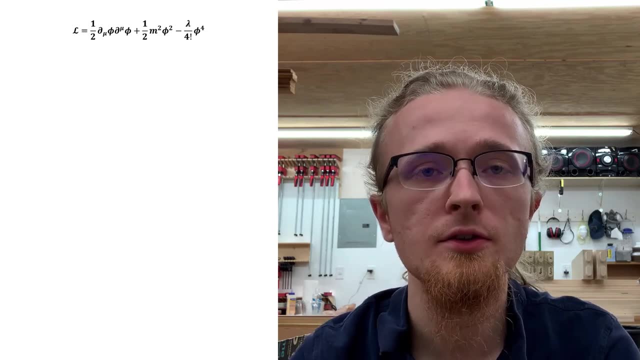 important feature is that the mass term has the wrong sign, which is equivalent to inserting an imaginary value for the mass into a theory with the normal mass term sign, ie the scalars or tachyons. A note on my notation here: In most textbooks the mass term has the wrong sign. 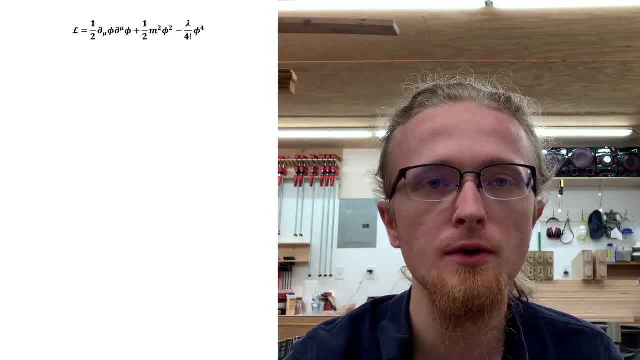 The mass term has the wrong sign. In most textbooks the mass term has the wrong sign. The mass term has the wrong sign. The mass term has the wrong sign. The normal sign will be written in the Lagrangian and the author will just tell you that the mass has. 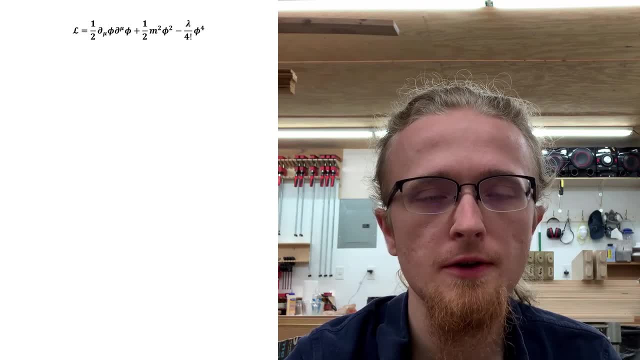 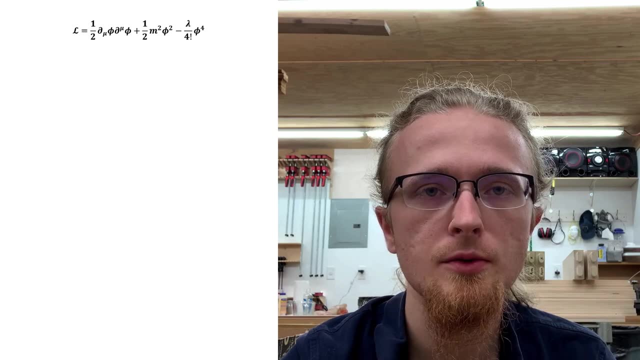 an imaginary value. I'm using the somewhat unusual convention of explicitly flipping the sign on the mass term and taking m to be real. I think this makes the math clearer. Anyway, continuing on The tachyonic mass term may seem like a great unphysicality in and of itself. 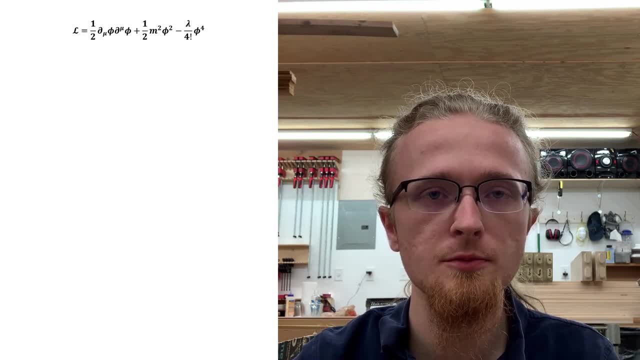 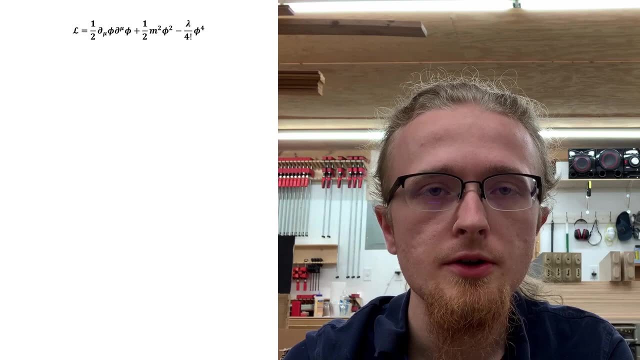 but due to something called tachyon condensation, which I'll discuss more later, it isn't necessarily a physicality deal breaker. There is, however, another subtler unphysicality in this theory, also resulting from the mass term having the wrong sign, and it turns out that fixing this 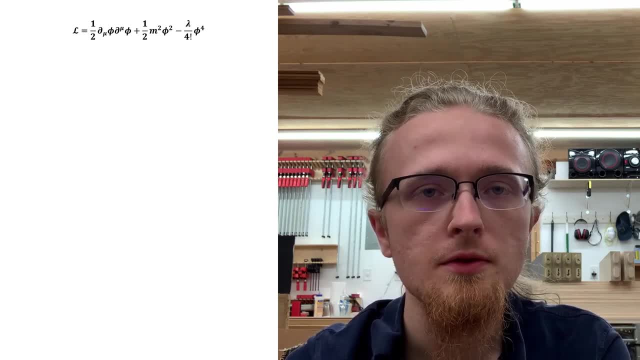 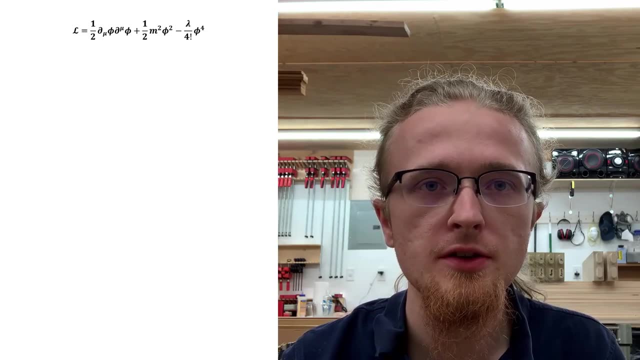 unphysicality is where things really start to get interesting. The fix is heavily connected with the sign inversion symmetry of the theory, which is eliminated by the fix at low energy. The fix to this subtler problem also happens to eliminate the tachyons at low energy. 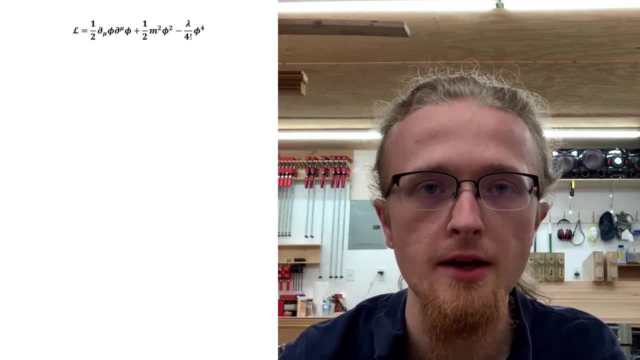 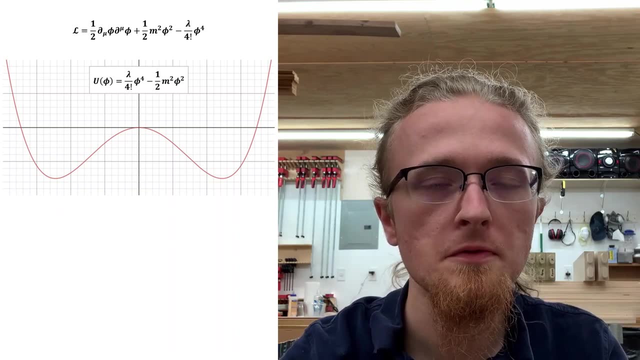 but we still rely on tachyon condensation to handle them at high energy. To see the problem we must graph the complete potential term from this theory, which includes the mass term. We see the famous Mexican hat shape with minima at plus or minus root, 6 m squared over lambda. 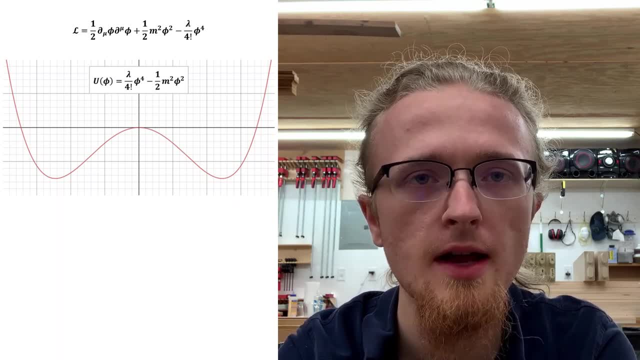 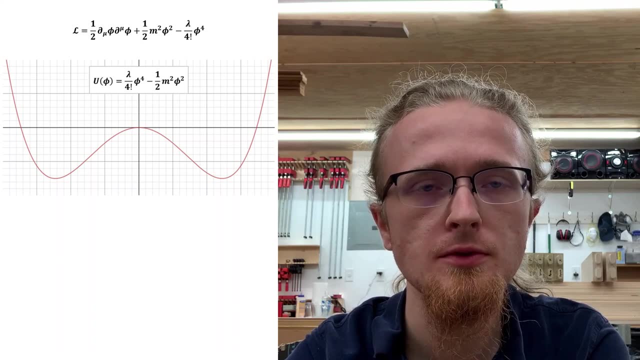 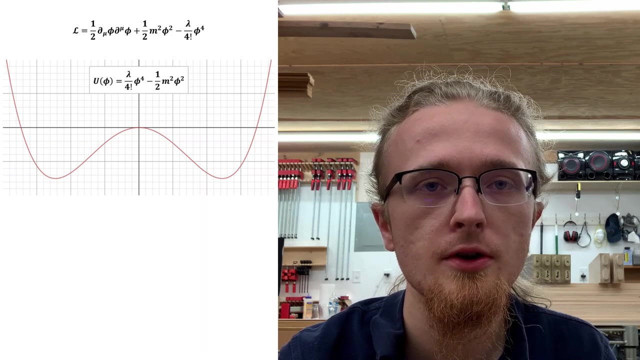 These minima serve as seemingly unphysical, non-zero, classical vacuum solutions to the theory. Notice that, while the theory overall is invariant, under sign inversion these vacuum solutions are not. However, the sign inversion transformation merely transforms one of the vacuum solutions into the other. 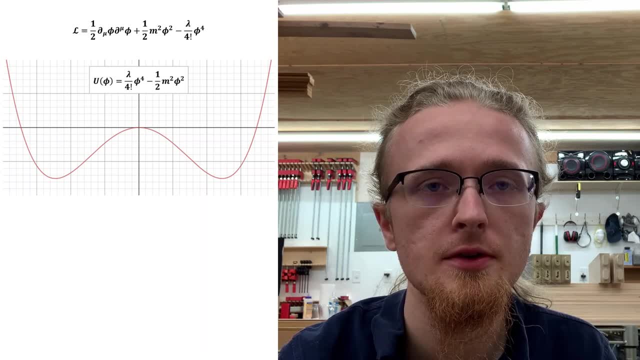 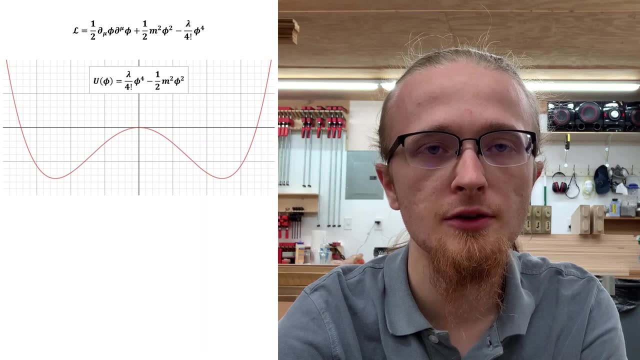 a reflection of the overall sign inversion symmetry of the theory. Let's think about this carefully. Above the middle bump, there is no feature in the potential to force the vacuum field to fluctuate asymmetrically about zero and, as a result, the vacuum expectation value is equal to zero. 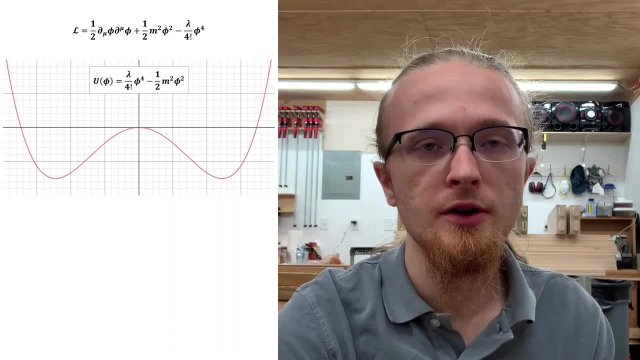 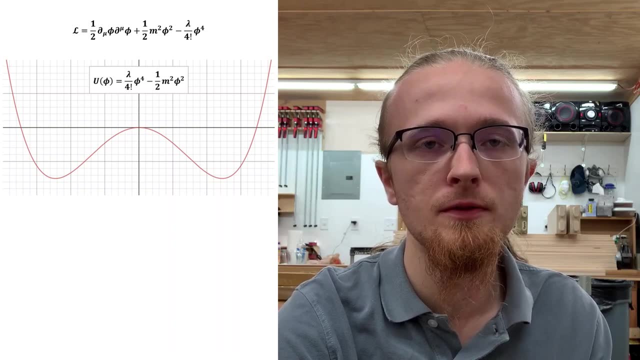 The theory is completely physical in this regard. However, when considering energy levels below the middle bump, while the potential is still symmetric, the middle bump forces the vacuum field to fluctuate about one of two non-zero values, resulting in a non-zero vacuum expectation. 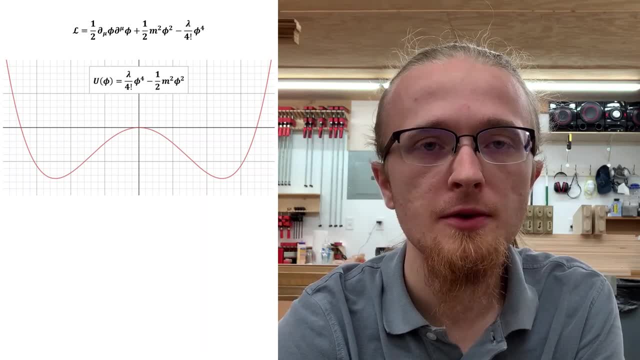 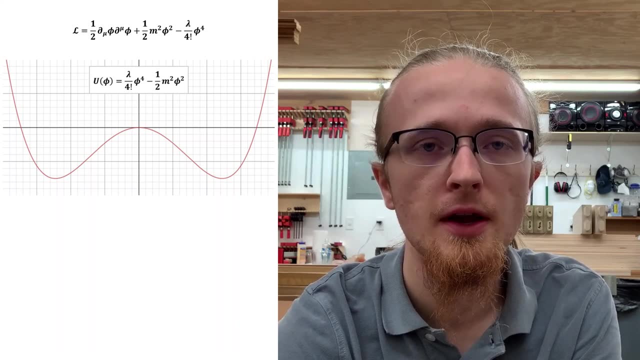 value which is clearly unphysical. We therefore have a theory that may be physical above a energy level, assuming that something else doesn't get in the way, but that is very much unphysical below that energy level. Here's where the magic happens: We can reparameterize the Lagrangian. 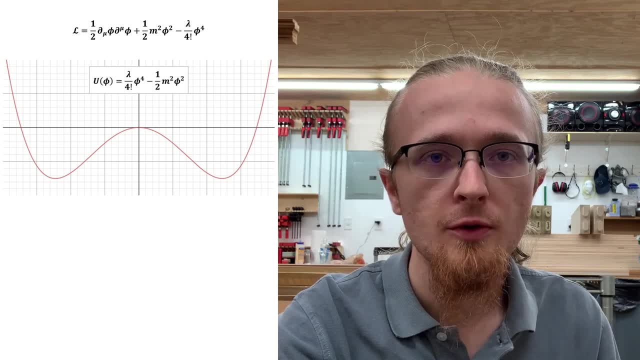 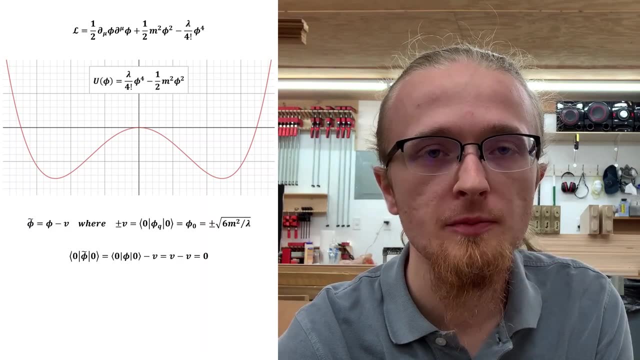 density, such that it turns into one with no such unphysicality, but where the sign flipping symmetry is no longer present. The parameterization that we need to accomplish this is this: Notice that the vacuum expectation value of this new field is zero, even below the bump height of 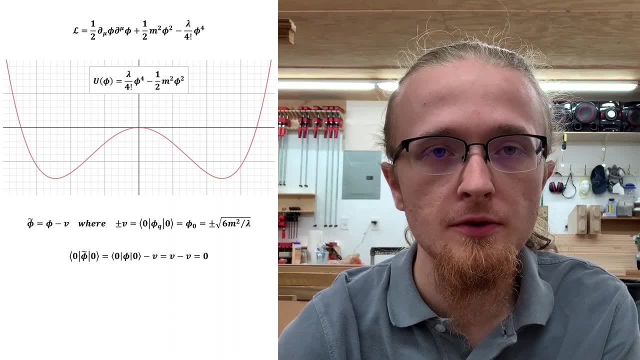 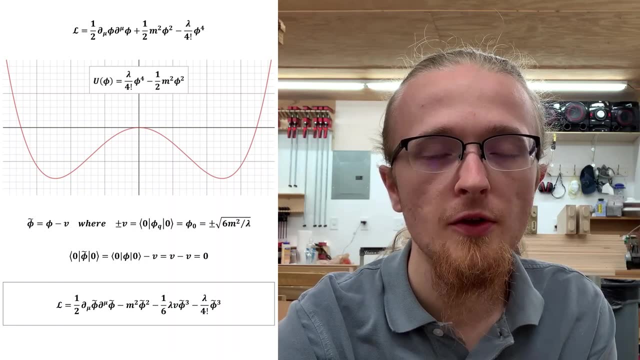 the original potential. Inserting this reparameterization yields this new Lagrangian density. Note that this Lagrangian density doesn't have the sign flipping symmetry that the one we started with had, but the sign on the mass term is no longer tachyonic and 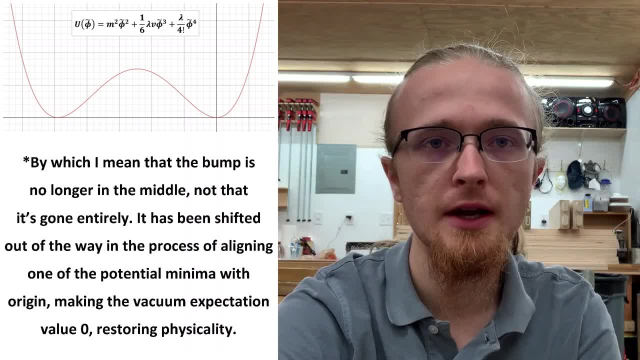 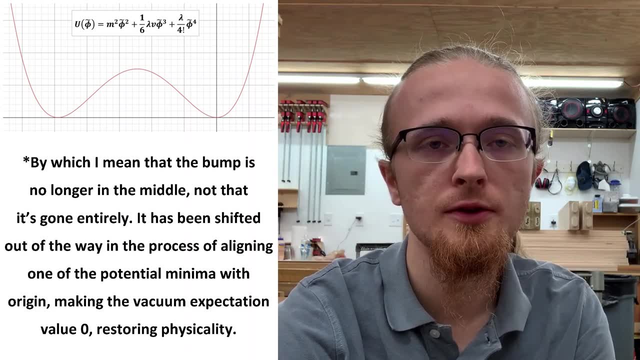 the graph of the potential function no longer has a bump in the middle. In short, we've gained physicality at the cost of the manifest symmetry, The general idea of restoring physicality below a certain energy level to a theory with a bump, or Mexican. 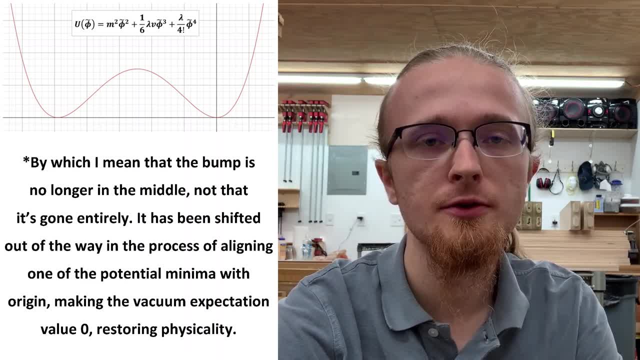 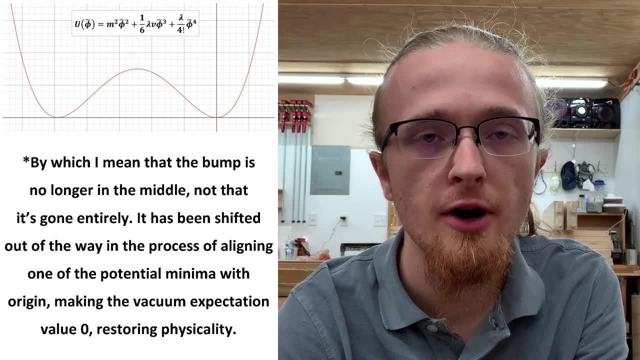 hat potential at the cost of symmetry via a shifted field. reparameterization is an important one in a broader context. This is because, when the Lagrangian density is changed, only by such a re-parameterization, many of the critical properties of the original action. 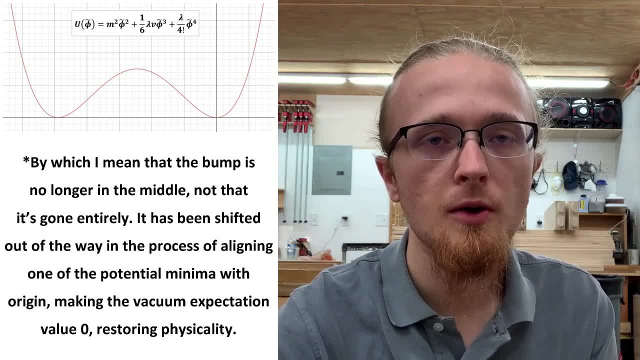 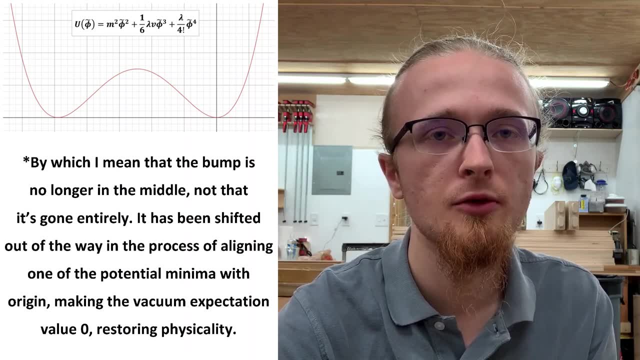 are often maintained. Sometimes you can find a Lagrangian density with one property that you like, for example its renormalizable. that can be re-parameterized into another Lagrangian density with a different property that you like, for example, maybe it contains. 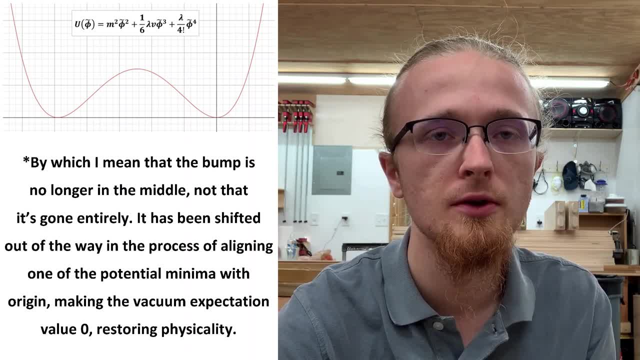 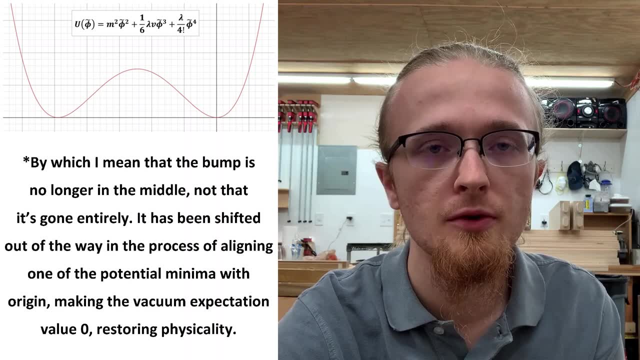 massive vector bosons without destroying the property that you liked about the original Lagrangian density. This is actually the idea behind writing a renormalizable theory of massive vector bosons via the Higgs-Kibble mechanism, which is employed in the Standard. 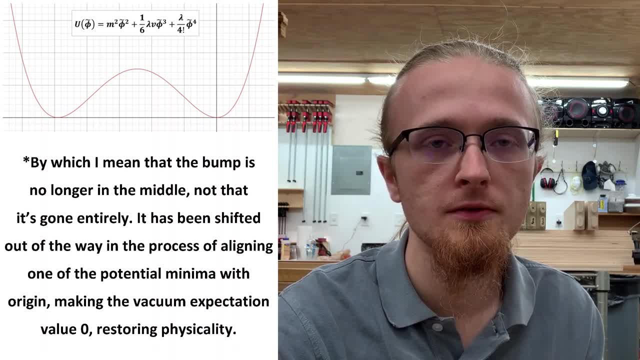 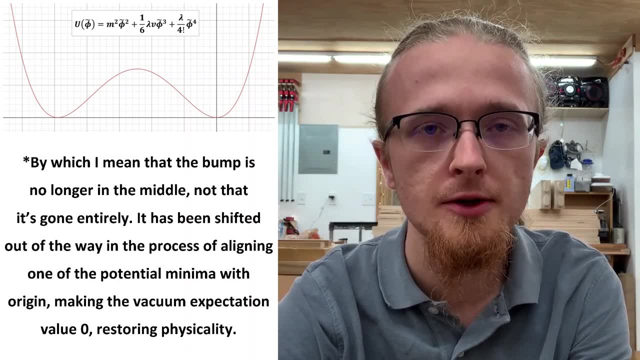 Model. In the Standard Model the Higgs field also gives mass to the fermions via Yukawa couplings, but we won't cover that in this video. One may ask about the unphysicality of a tachyon field at high energy in a theory used for phenomenology. It turns out that 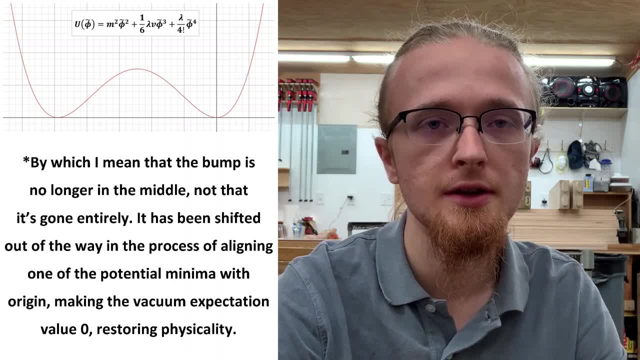 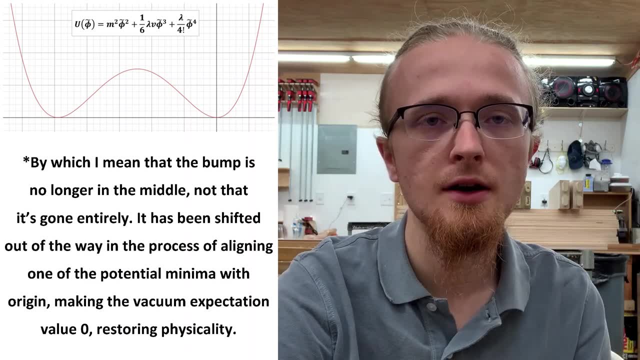 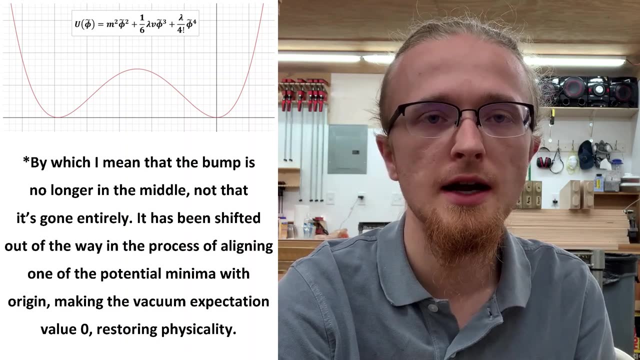 configurations involving tachyonic excitations are innately unstable and always decay into configurations involving no real tachyons. This is the process of tachyon condensation. Therefore, using a tachyonic field to break symmetry doesn't imply unphysicality at high. 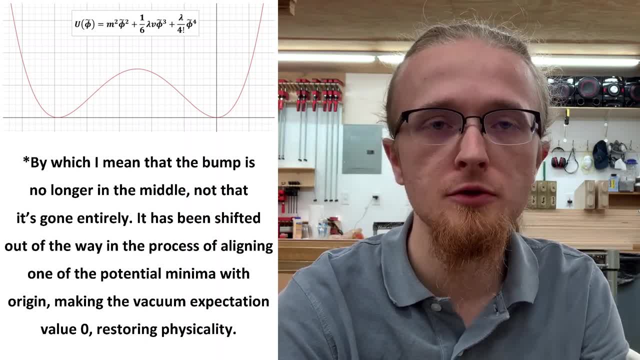 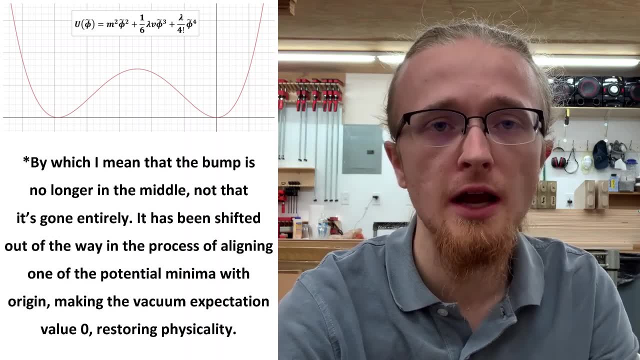 energy. With that simple example in the bag, let's move on to a more sophisticated analog of that problem and then apply the knowledge that we gained from handling that more sophisticated analog to still another example that demonstrates the Higgs-Kibble mechanism, or Higgs mechanism. 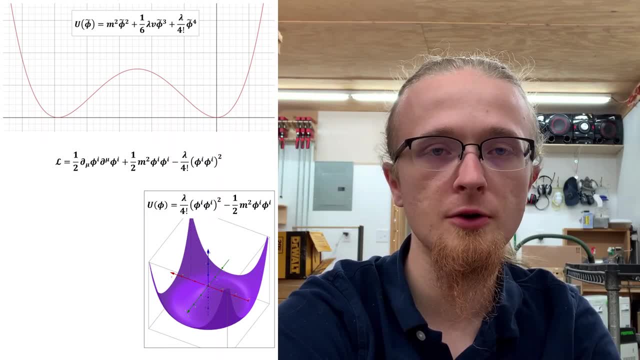 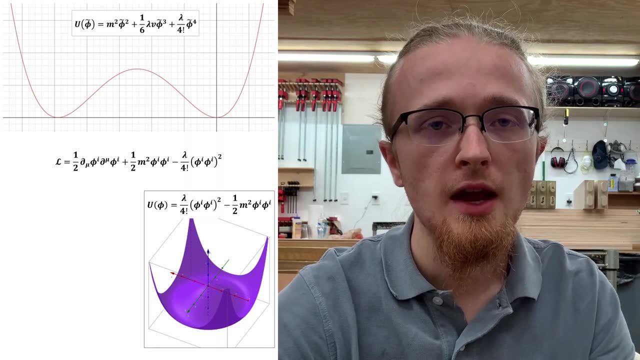 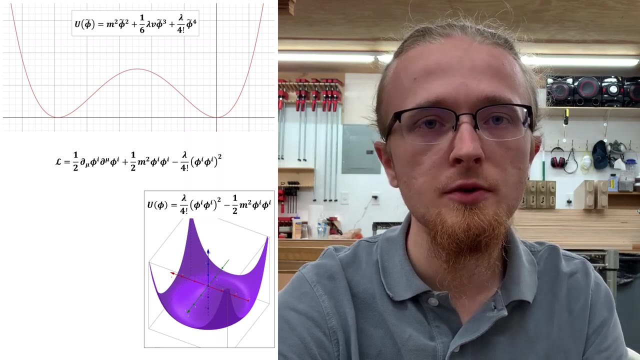 for short. This second theory we're going to consider is given by this globally ON symmetric Lagrangian density, We again see that we have a set of non-zero classical vacuum solutions and an unphysical, non-zero vacuum expectation value at low energy. in the quantized theory, Specifically, we 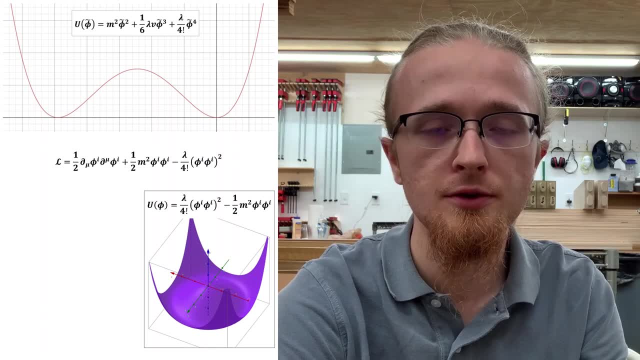 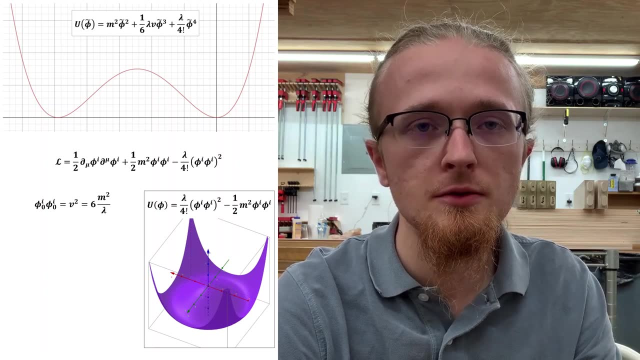 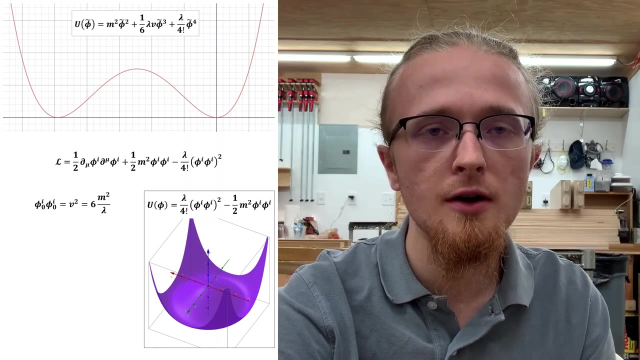 have a degenerate ring of non-zero classical vacuum solutions sitting at the bottom of the potential solving this equation, Similar to the example we just handled. these vacuum solutions aren't invariant under the complete ON symmetry group, but they're transformed into other valid solutions when acted upon. 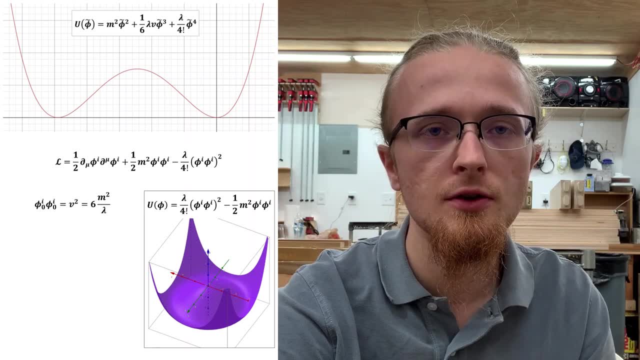 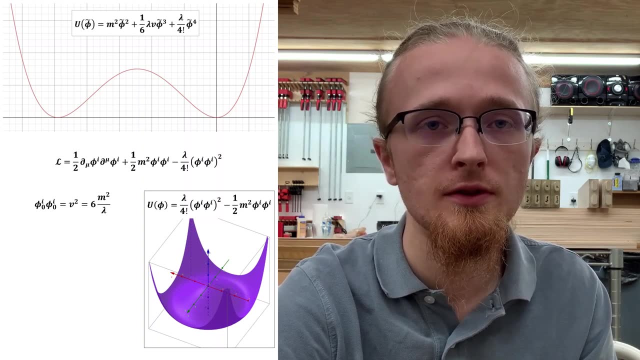 by ON transverse, They're not invariant under transformations under which they're not invariant. so the overall theory remains invariant. Because all of these classical vacuum solutions are degenerate, we may as well select one that's easy to work with for further consideration. 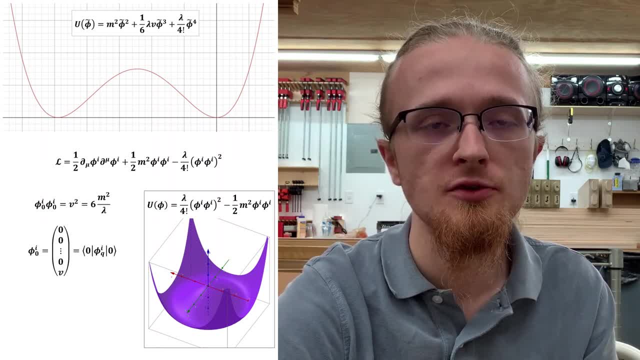 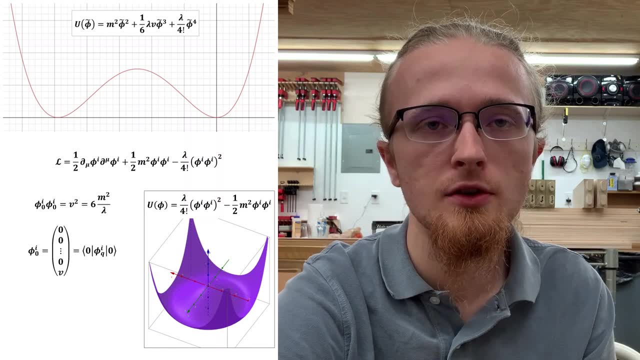 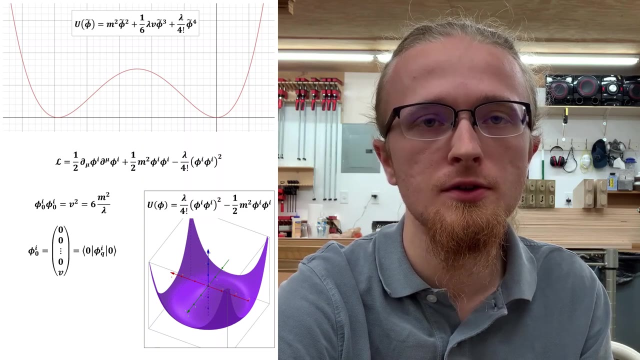 The standard selection singles out the specific direction in ISA's spin space corresponding to the last component where, just to be clear, phi i is the classical field and phi qi is the corresponding quantum field. This vacuum solution is of course not invariant under the complete ON group, but it is invariant. 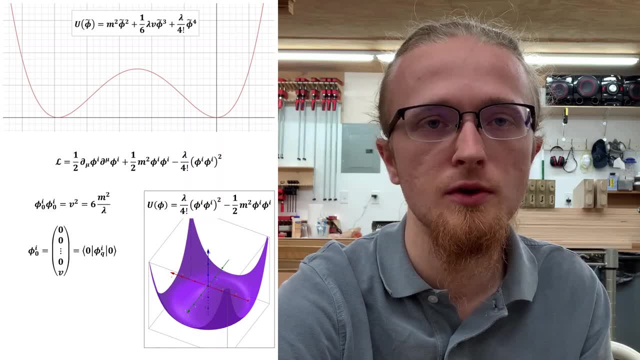 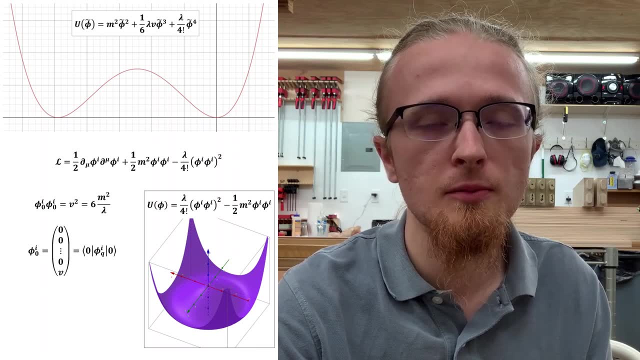 under all transformations that don't affect the last component. This obviously amounts to ON-1 symmetry. Therefore, if we do something similar to what we did in the last example and expand around this vacuum solution as our reparameterization aimed at restoring physicality, we'll end. 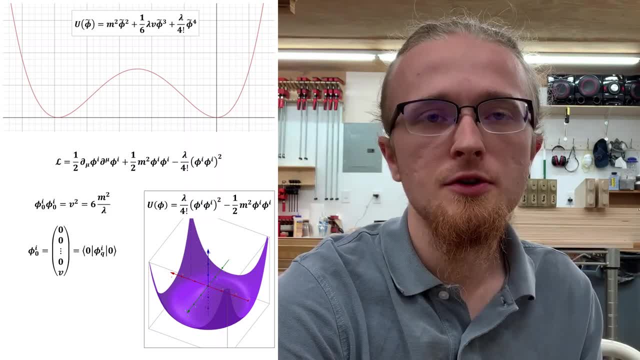 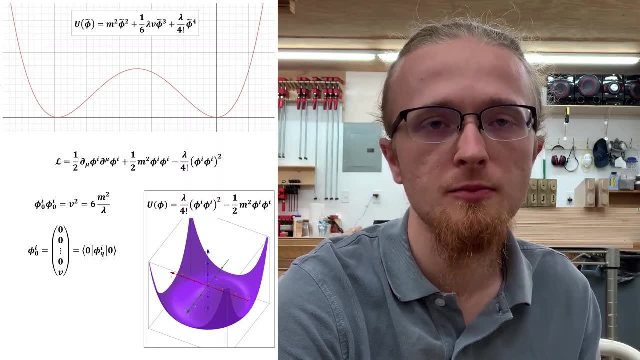 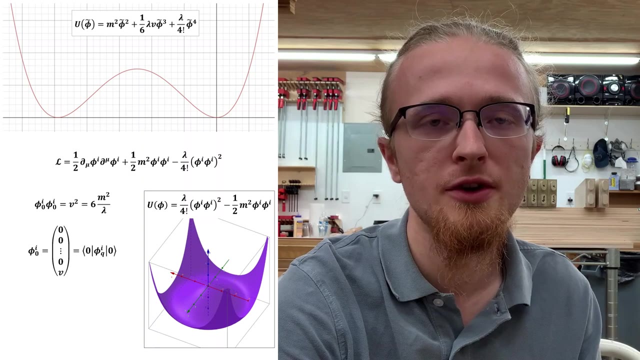 up with an ON-1 symmetric theory. Such a potential shift has this effect because we're only shifting the last component of the field, which corresponds to shifting the potential out of a symmetric position in only one direction in ISA. The resulting potential is therefore symmetric in all other directions in ISA's spin space. 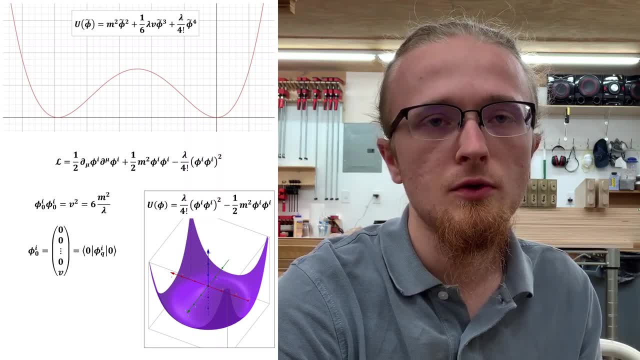 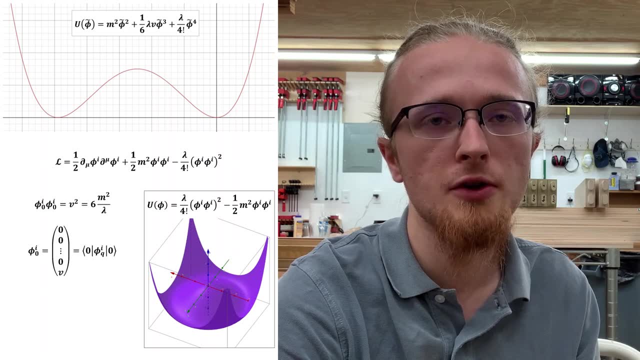 As it happens, the reparameterization that we're actually going to use only leaves a potential for the field in the last component, so the potential is definitely invariant under ON-1 transformations of the other fields. We're not going to use exactly the same reparameterization that we did in the last example, because that 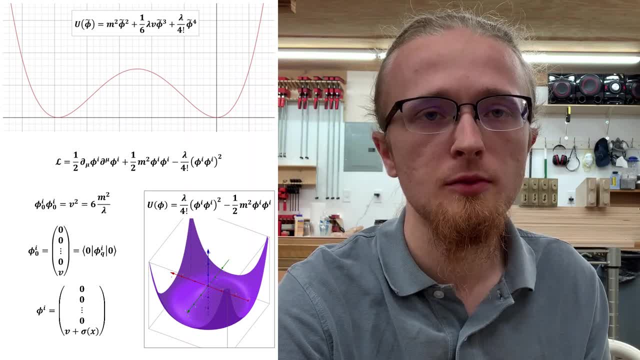 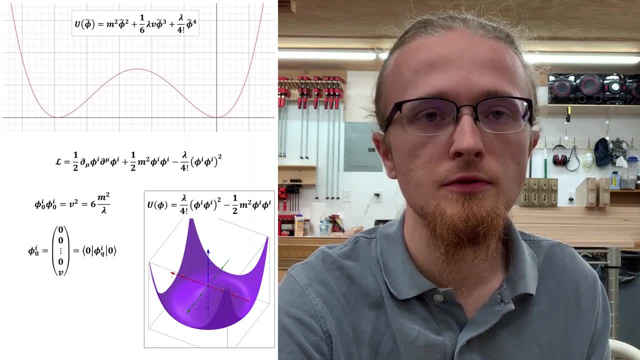 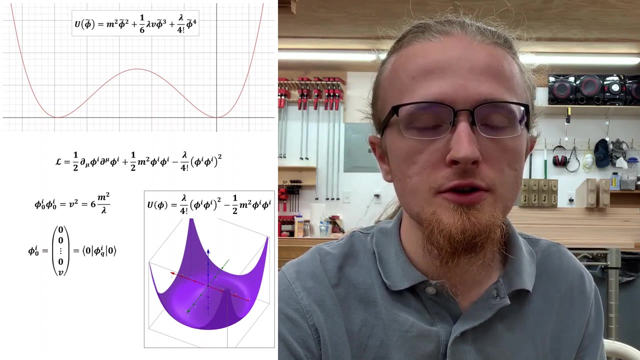 would result in a theory with only one field in it coming from the last component, and that's not very interesting. Instead, we'll use a different reparameterization that also represents expanding around this vacuum, but involves more fields. In short, because the amount of symmetry in the second example, Lagrangian, is so much greater. 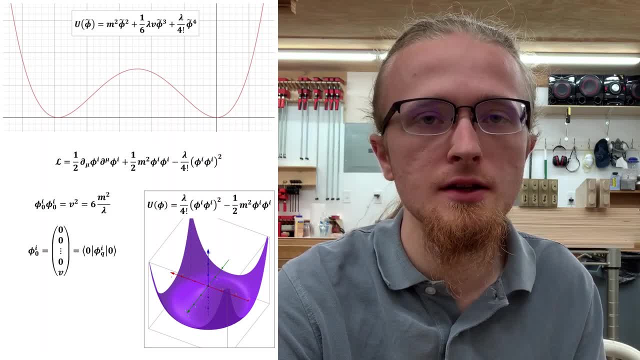 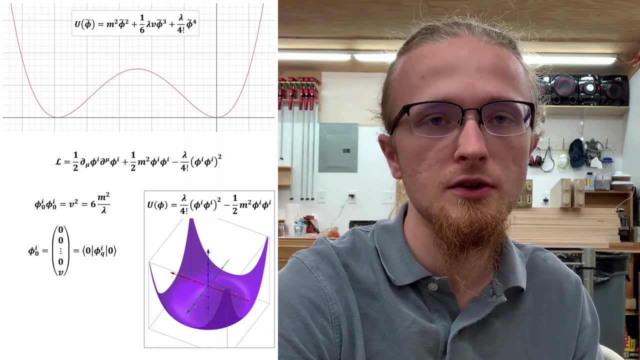 we don't have to sacrifice all of it in order to restore physicality in a theory with essentially the same potential To break all of the symmetry, one would need to select a potential with classical vacuum solutions that are completely unsymmetrical. This trend of only needing to break the symmetries under which the vacua are not symmetric in 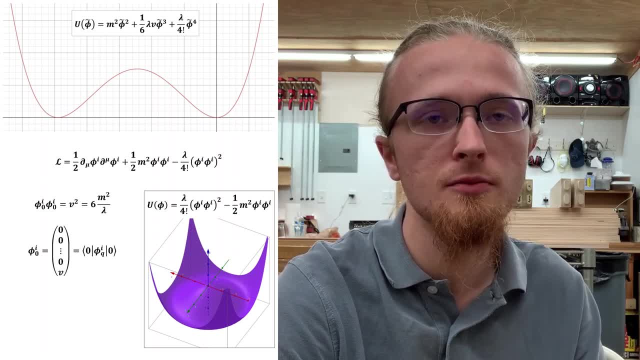 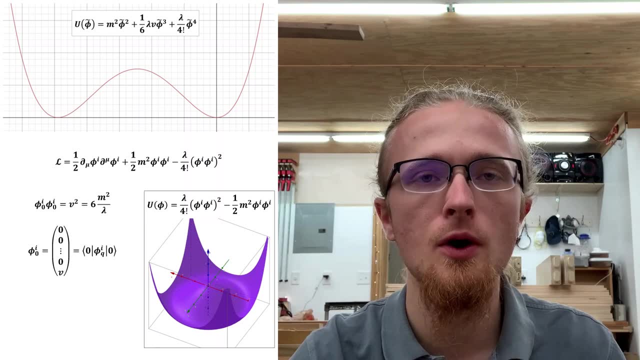 order to restore physicality is a fundamental one, and one that we should pay attention to going forward. Let's now actually do this. Let's break the ON symmetry of our Lagrangian down to ON-1 symmetry via a reparameterization of the fields. 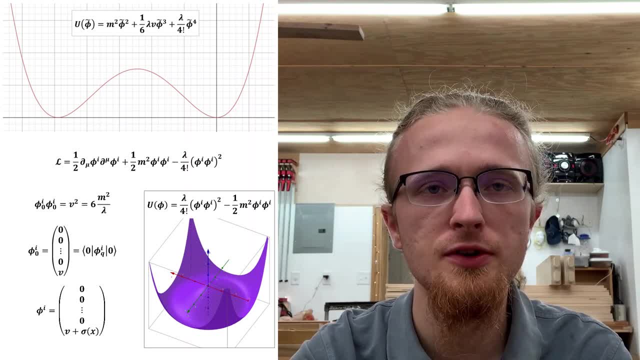 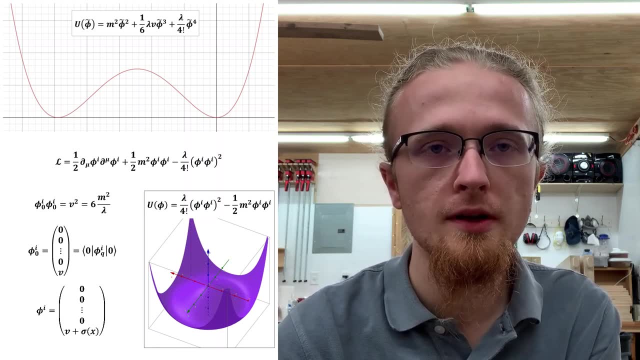 The most obvious choice is the direct analog of what we used in the first example. but, as I mentioned a little bit ago, this doesn't yield a very interesting theory because it replaces N fields with just one. In principle, we can have as many independent fields in the reparameterization as there. 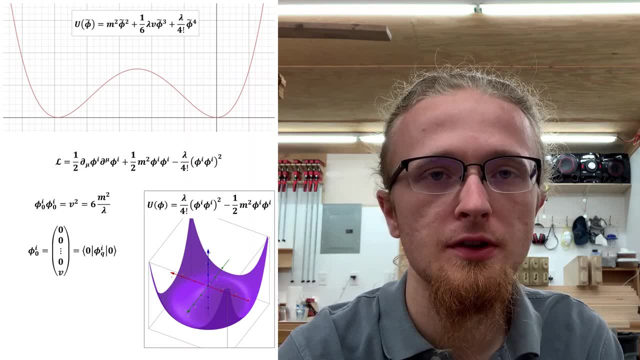 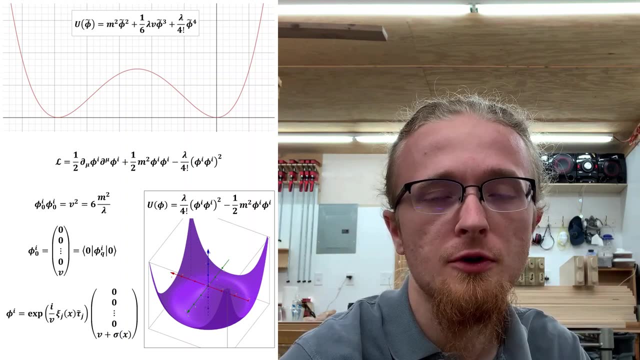 are in the original theory. Partly because of this, a much more interesting theory is yielded by this more complicated reparameterization, where J runs from 1 to N-1, and superscript I and later K run from 1 to N. 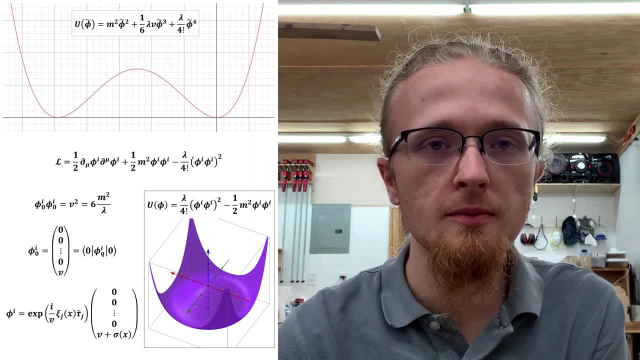 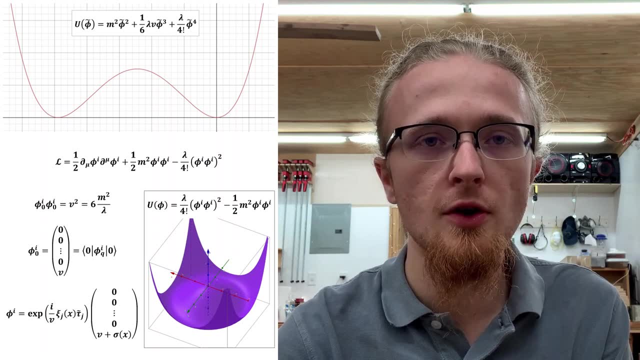 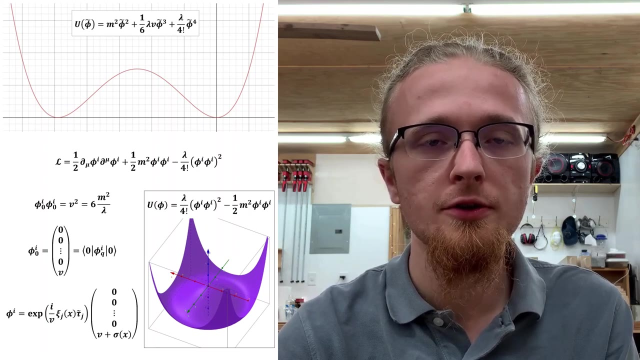 Tau-tilde is the set of ON generators that are not also ON-1 generators. They're usually called broken generators because they generate the symmetry transformations under which the resulting theory is not invariant. This more complicated reparameterization includes the shift that I was talking about, but it also includes an arbitrary local ON transformation that. 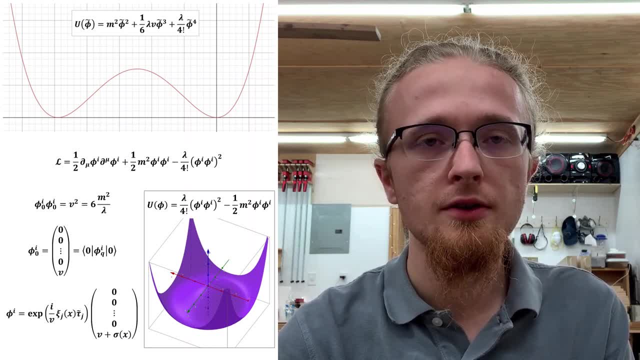 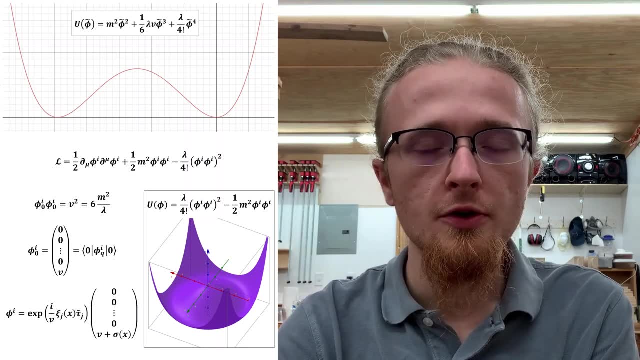 is not in the ON-1 subset. This extra factor doesn't affect the shifting of the potential because the entire potential term is locally invariant under all ON transformations. Also, we have a total of N fields in this reparameterization sigma and the N-1 xi fields. 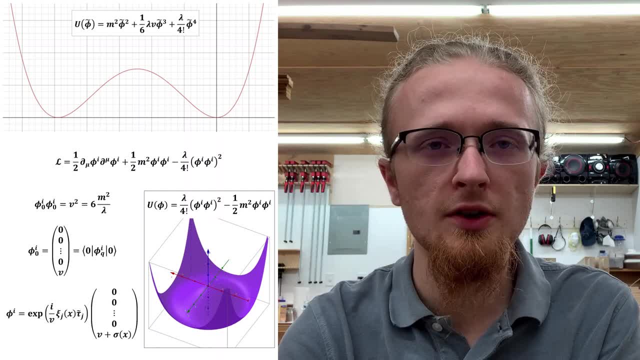 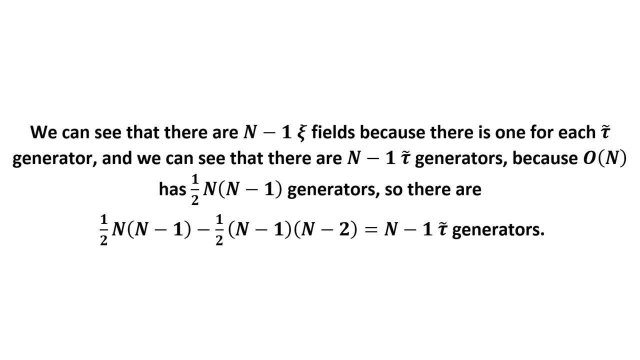 At least I think that Greek letter is pronounced xi, maybe it's xi, I don't know. We can see that there are N-1 xi fields, because there's one for each tau-tilde generator, and we can see that there are N-1 tau-tilde. 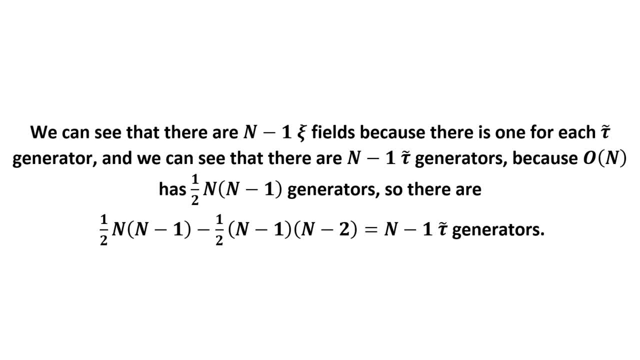 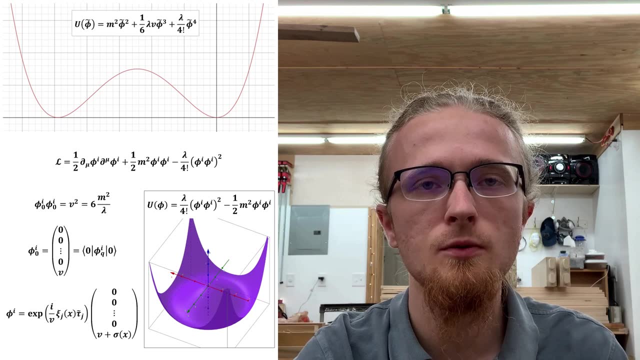 generators, because ON has a half N times N-1 generators, So there are one half N times N-1, minus a half N-1 times N-2, or N-1 tau-tilde generators. This reparameterization is therefore an elegant way of including all the fields we need without 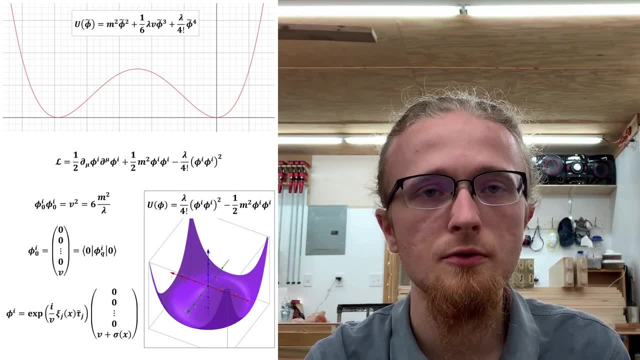 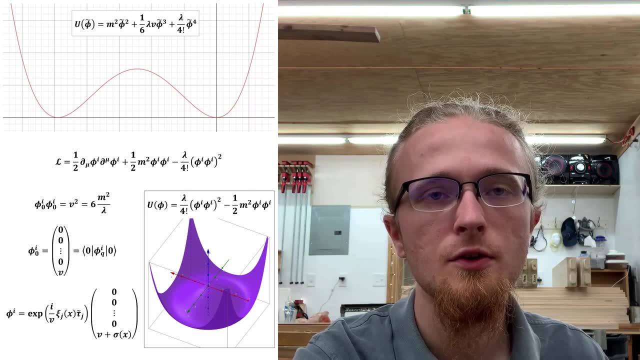 disrupting the shifting of the potential. The other reason for selecting this reparameterization is that it yields a very physically sensible theory in a way that I don't want to use in this video, so I'm going to go ahead and do that. The fact that it generalizes so well to other theories involving spontaneous symmetry breaking 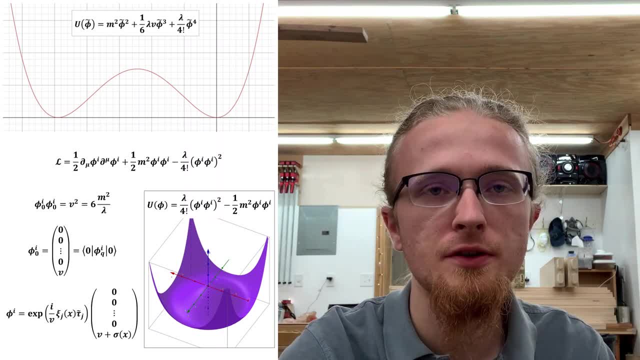 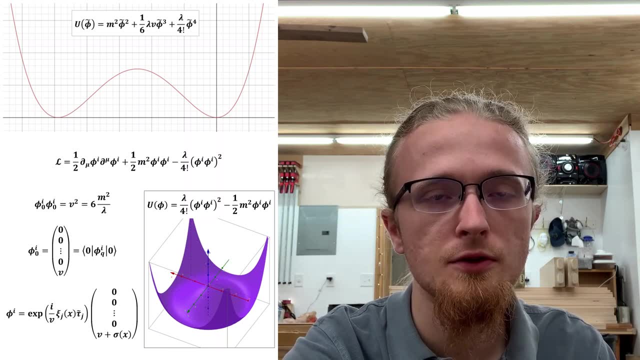 is one of the reasons why it's selected. The field quanta given by the xi fields are called Nambu goldstone bosons, And when applying a reparameterization of this form to the general case, you always need as many Nambu goldstone boson fields as you have broken generators. 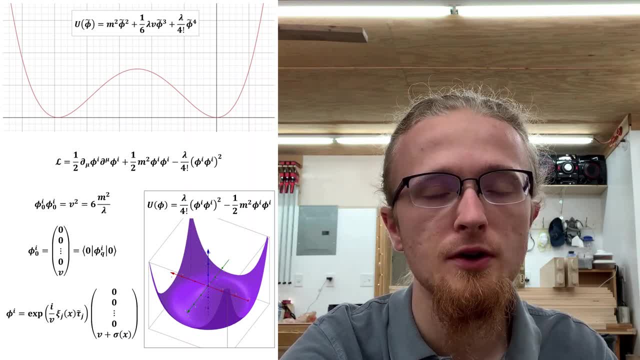 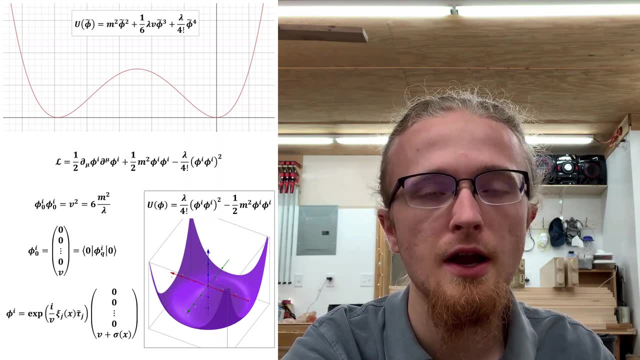 The fact that there are as many broken generators as there are unbroken directions in isospin space is called the goldstone theorem. It's often simply summarized by saying that the resulting theory has one Nambu goldstone boson for every broken generator. 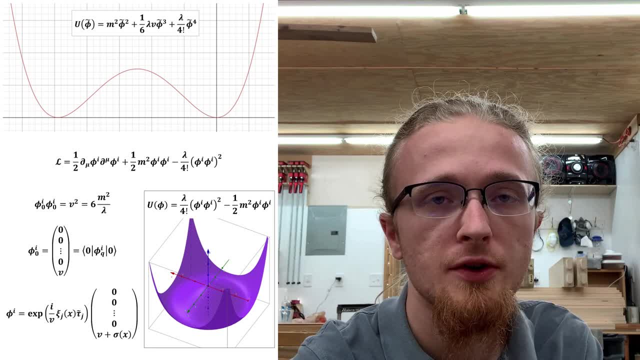 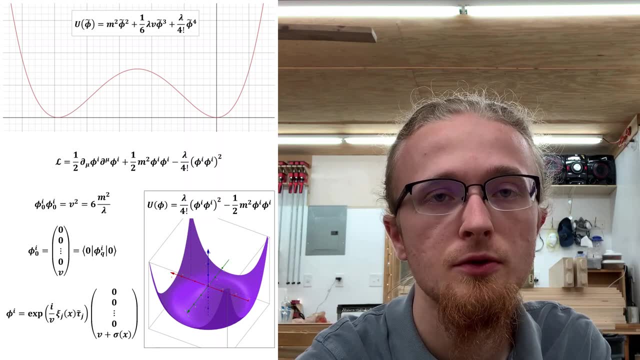 I'm not going to prove the goldstone theorem in this video, but we will discuss Nambu goldstone bosons further. However, it's useful to have the spontaneously broken Lagrangian density in hand when we do that. so let's work that out first. 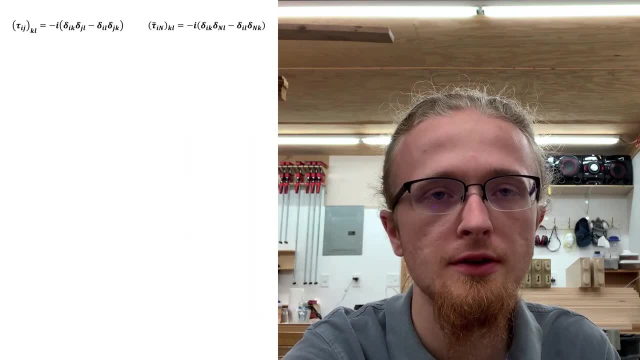 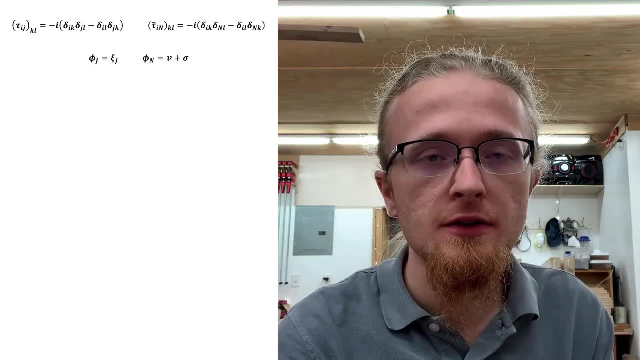 The most useful formulas for the generators in this application are these Kronecker delta expressions. With those expressions to lowest order, we see that the fields have these values. Finally, we see that the fields have these values. Finally, inserting the parameterization produces this spontaneously broken Lagrangian density. 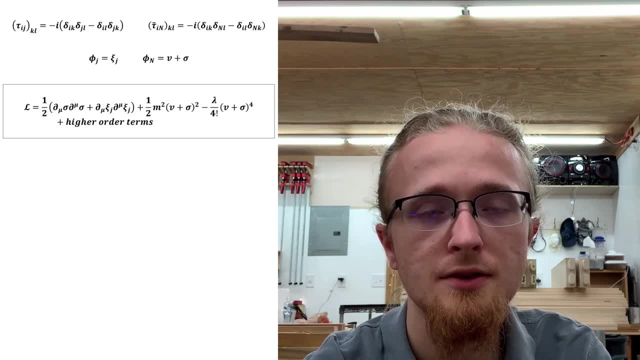 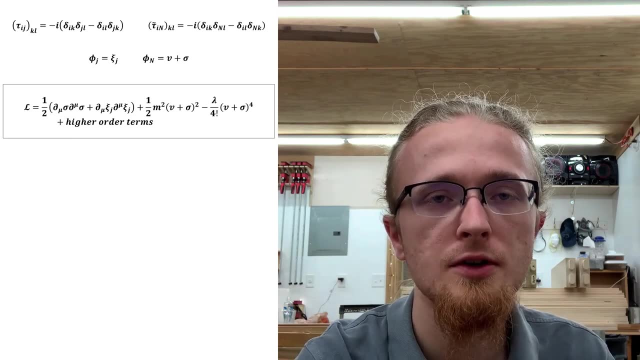 Looking at this Lagrangian carefully, we see that the sigma field is massive and not tachyonic, and we also see that the Nambu goldstone bosons are not massive. As part of our discussion of shifting the potential, we already noted that the factor 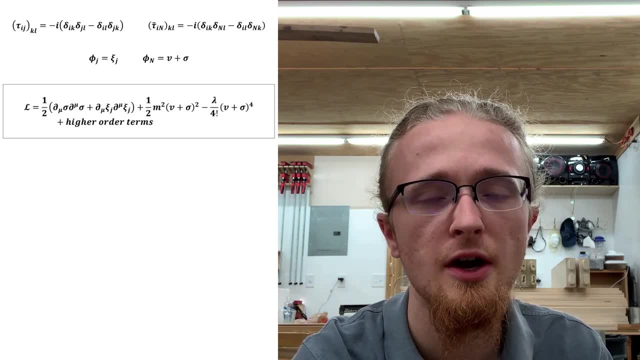 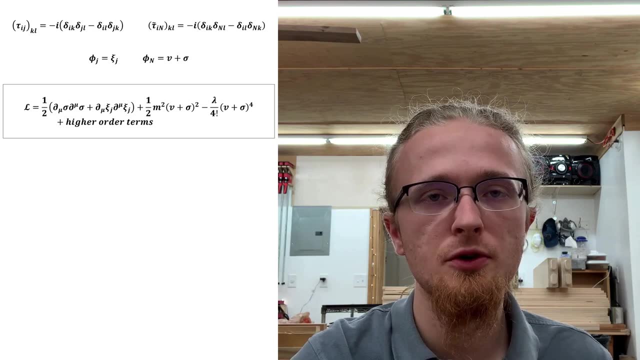 carrying the Nambu goldstone bosons is an invariance of the entire potential term, including the mass term. As a result of that decoupling from the mass term, it's no surprise that the Nambu goldstone bosons turned out to be massless. 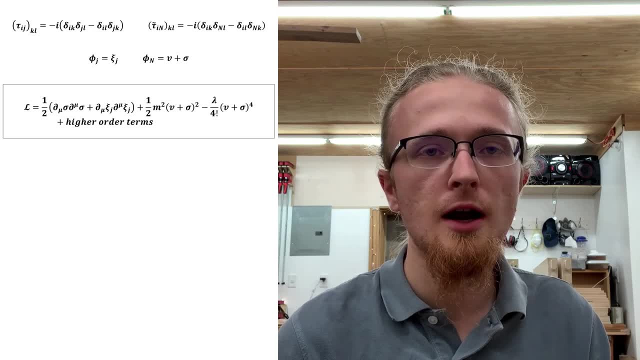 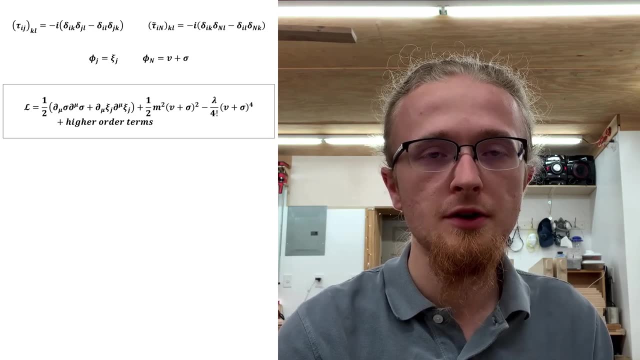 The Nambu goldstone bosons are often said to be the modes running around the circle at the minimum of the potential, because they're associated with the unbroken directions in isospin space. The mass of sigma boson is said to be running perpendicular to the ring at the bottom of 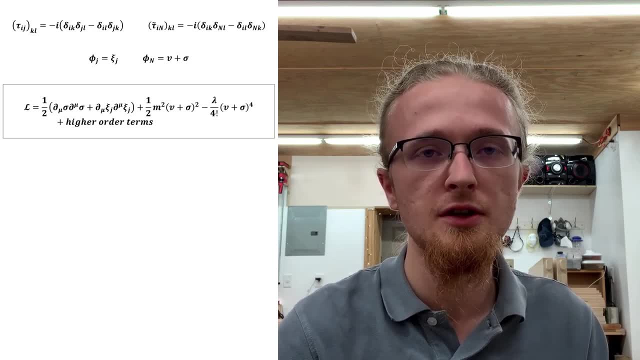 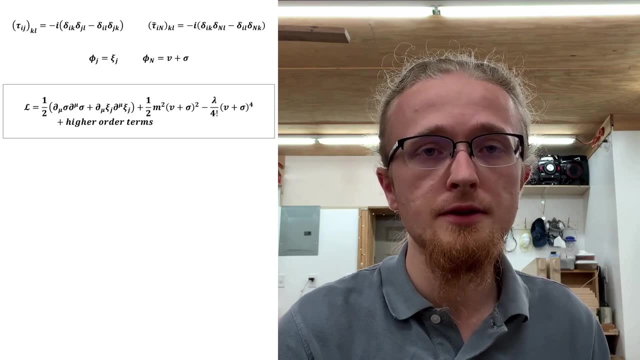 the potential and acquires its mass from the fact that the potential is in its way. It's worth noting that a lot of the words in that description are to be taken as an analogy rather than literally, if that wasn't obvious. All of these features are naturally general to theories with such a scale, so it's a 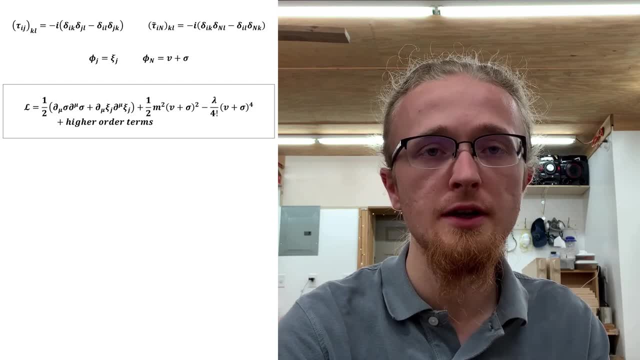 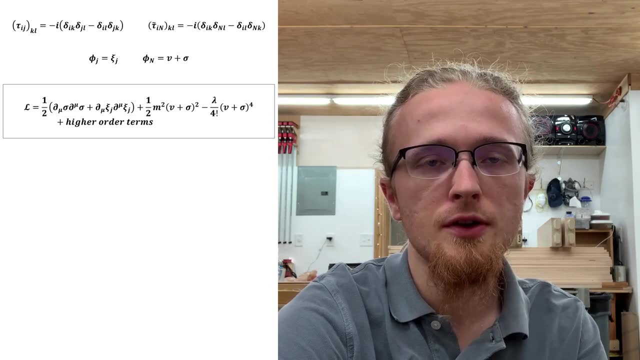 good idea to take a look at them, Thank you. So now that we've been introduced to the basic concept of spontaneous symmetry- breaking by the first example- and to Nambu, goldstone bosons and the Goldstone Theorem, by the second example- let's move on to the Higgs-Kibble mechanism, or the Higgs mechanism for short. 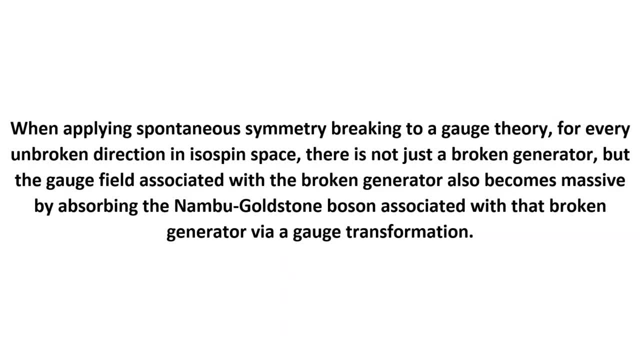 The basic addition to what we already know is as follows: When applying spontaneous symmetry breaking to gauge theory, for every unbroken direction in isospin space there is not just a broken generator, but the gauge field associated with the broken generator also becomes massive. 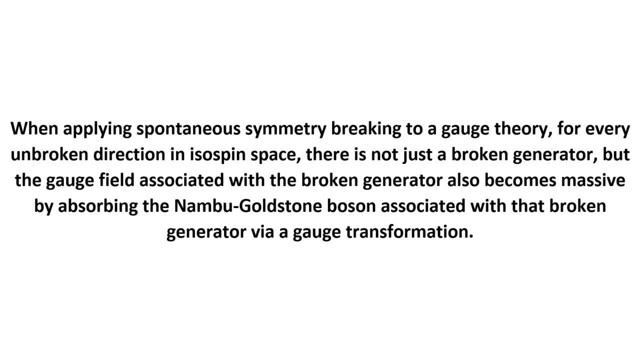 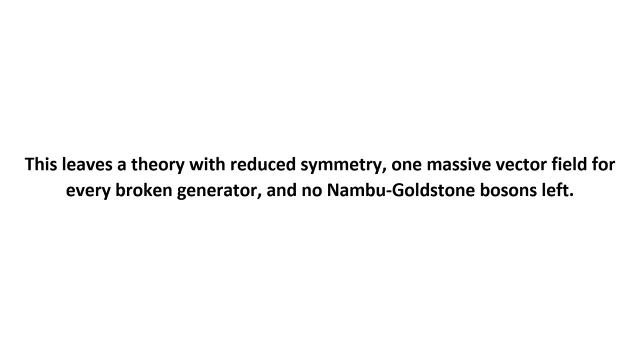 absorbing the name-bue goldstone boson associated with that broken generator via a gauge transformation. This leaves a theory with reduced symmetry, one massive vector field for every broken generator and no name-bue goldstone bosons left. Consider this U gauge theory. This is basically. 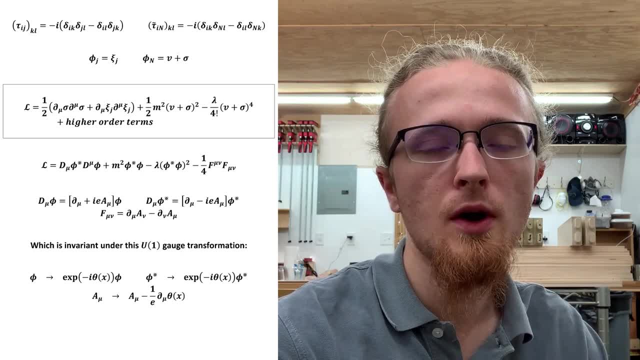 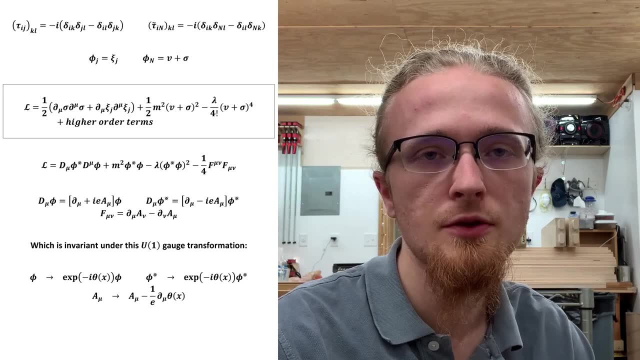 just scalar QED with Higgs potential set up to break the U gauge symmetry. Given that potential, the scalar classical vacuum solutions slash. possible vacuum expectation values are these: This is the natural analog of the reparameterization that we used in the second example, where the root 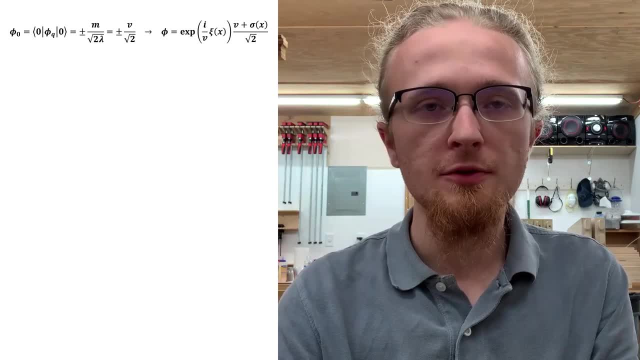 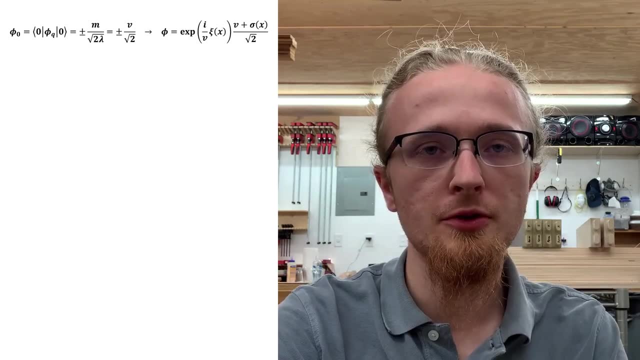 2 is just a conventional rescaling of the field. One might expect that the first factor in this reparameterization wouldn't even matter, because the entire theory is gauge-invariant. This reparameterization on its own, however, doesn't involve a transformation of the gauge field. 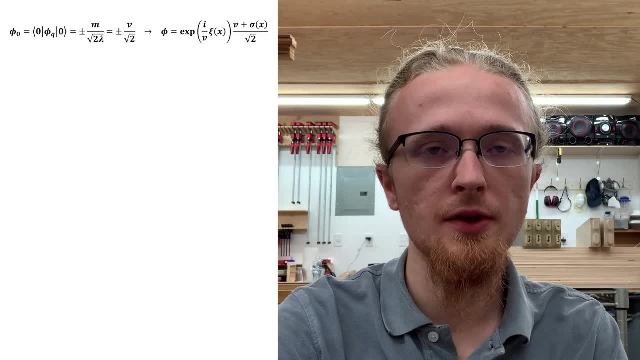 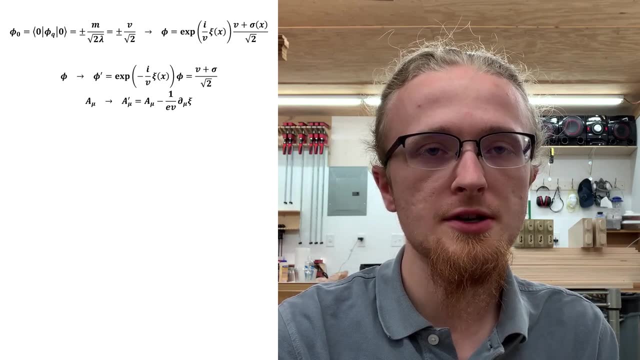 so it's effectively an incomplete gauge transformation. So with nothing but the insertion of this reparameterization, the Lagrangian would change. We can then perform an actually complete gauge transformation. The Lagrangian transforms the name-bue goldstone boson into the previously. 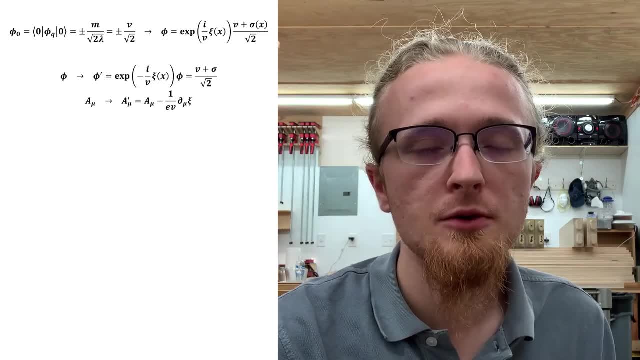 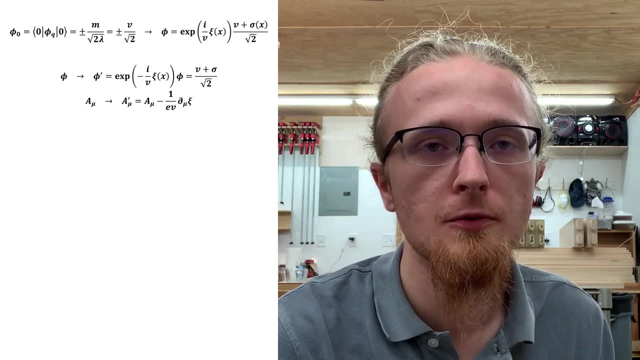 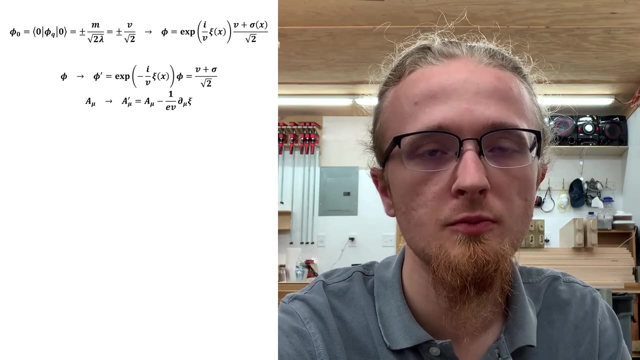 massless vector gauge field, making it massive For maximum convenience. we'll actually reverse these steps by first gauge transforming the Lagrangian and then inserting the gauge transformed field reparameterization into that. Looking at these gauge transformations you can see how they absorb the name-bue goldstone boson into the gauge field, And also for this: 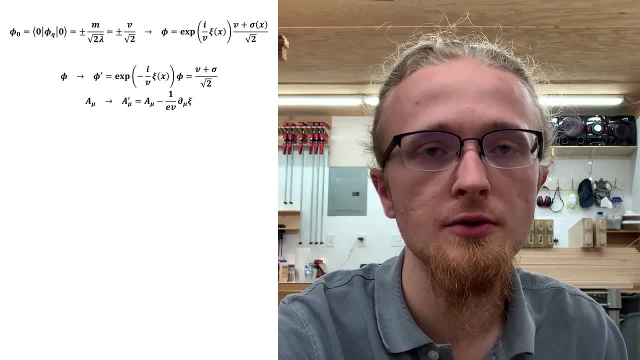 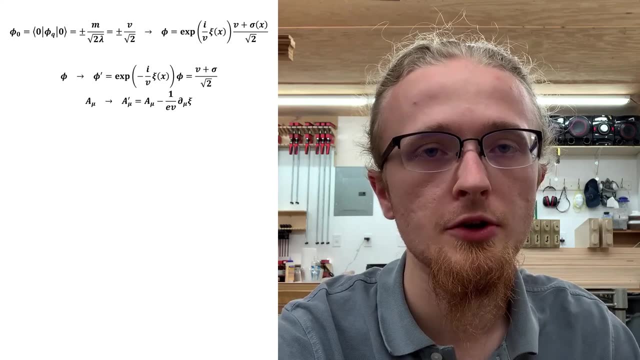 case I'll actually be showing all the algebra steps. I figure I ought to do it for at least one example, so I picked the most important example, the one that actually demonstrates the Higgs mechanism. So here goes: Given that the original Lagrangian density is gauge-invariant. 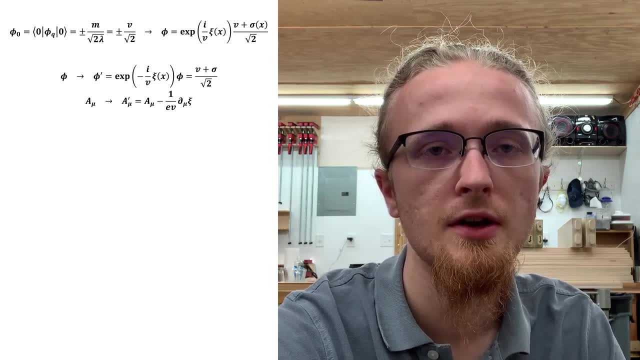 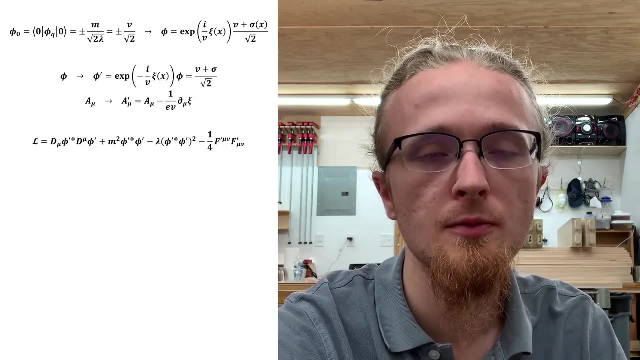 it doesn't change in form under our gauge transformation. so our gauge-transformed Lagrangian density is just this. If we then insert the gauge-covariant derivatives and the gauge-transformed field reparameterization, we arrive at this result. We can then pull out. 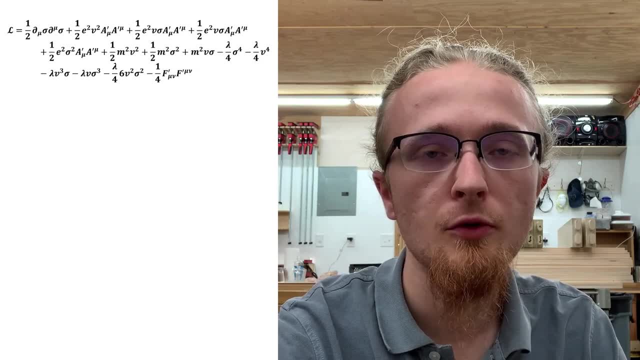 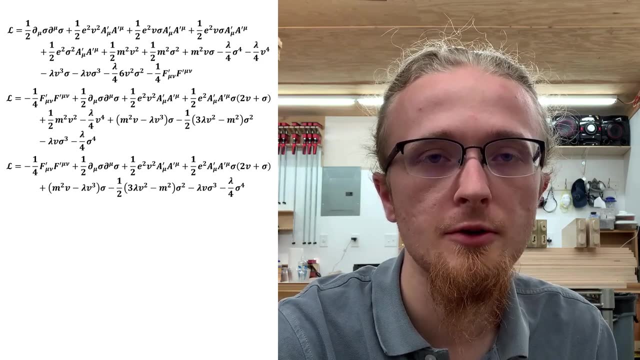 the factors of one over root, two and distribute. At this point we can see that several terms can cancel. We can then refactor the Lagrangian to yield this. We can also ignore the constant terms, because constant terms in the Lagrangian density don't amount to anything. Then finally, 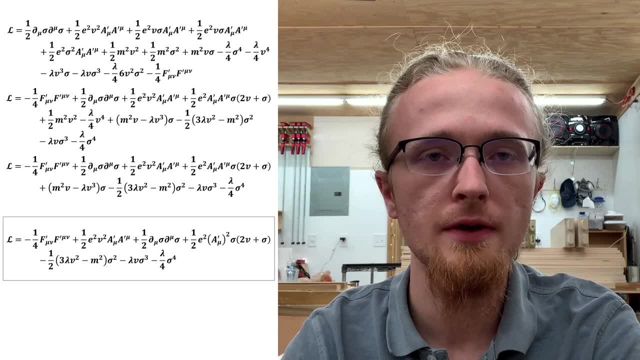 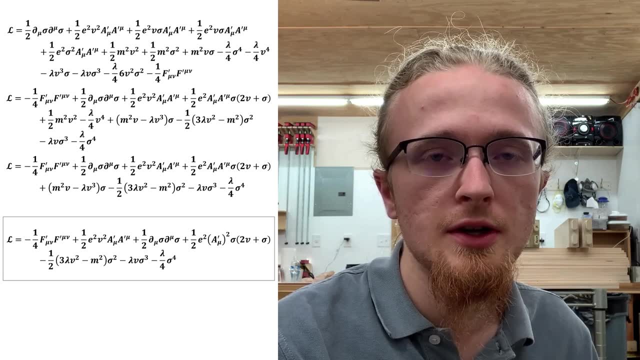 if we insert the value of v into the linear term, we see that it vanishes And with that we have our final, spontaneously broken Lagrangian density. Looking at this Lagrangian density, we see that the scalar boson is massive but not tachyonic. The vector field, which was 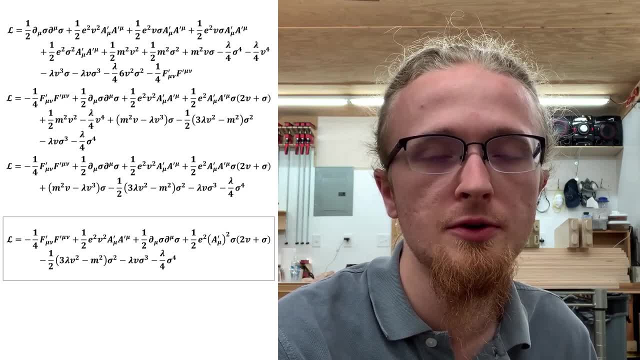 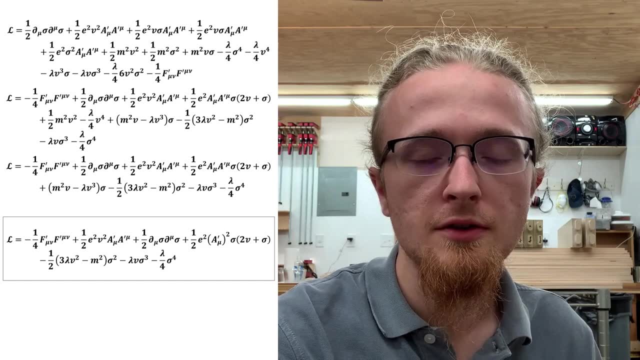 massless is now massive, and there are no name-bue goldstones to be found. This is the Higgs mechanism itself, in this case as applied to scalar QED, And this makes a whole lot of sense. Massless vector fields only have the two transverse modes, but massive ones have three. 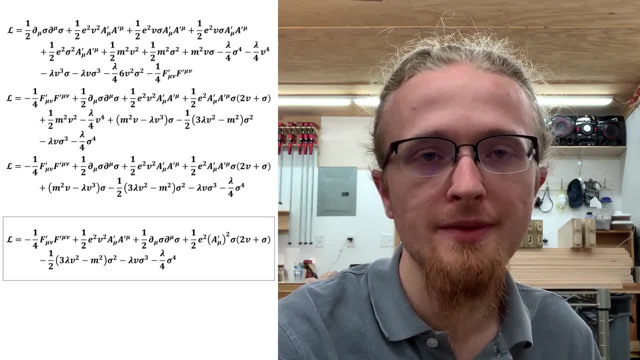 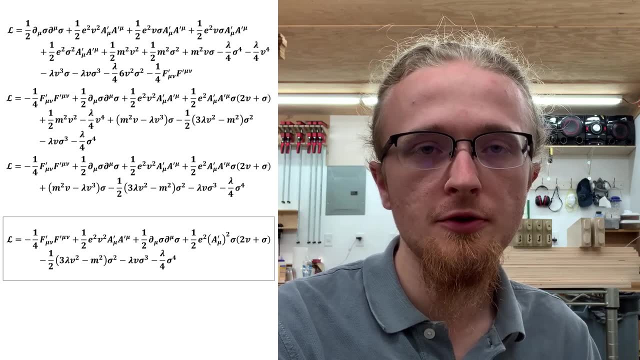 The name-bue goldstone boson that got absorbed into the formerly massless gauge field serves as that third mode. The vector field becoming massive also makes sense from a gauge theory perspective. A mass term for the gauge field explicitly violates gauge invariance. but once